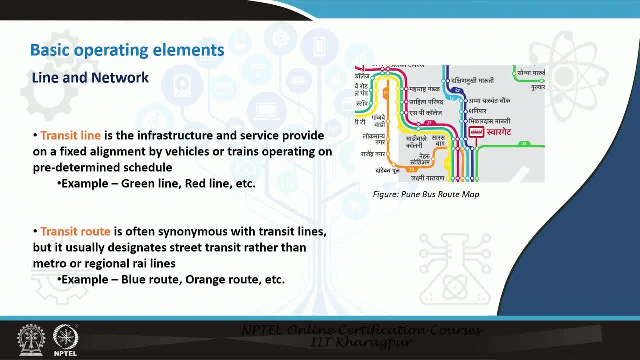 So how do we define a public transportation line? Ah, it is the infrastructure and service provided on a fixed alignment by vehicles or trains operating on predetermined schedules. So these are ah vehicles or trains operating on predetermined schedule and on a fixed alignment. 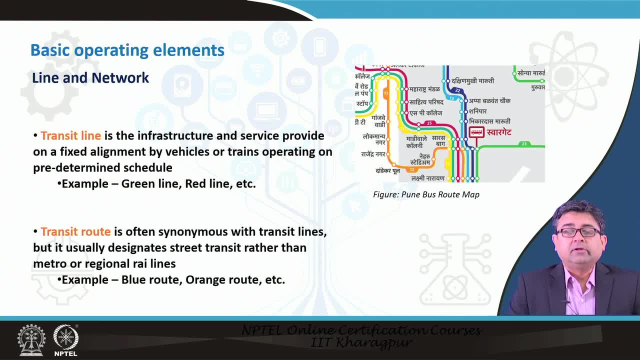 is: ah, you can see in the picture given on your right side that there are several different lines that you can take to go from point A to point B, such as yellow line, green line, red line, so on and so forth. So this is an example from the ah Pune bus route map. So 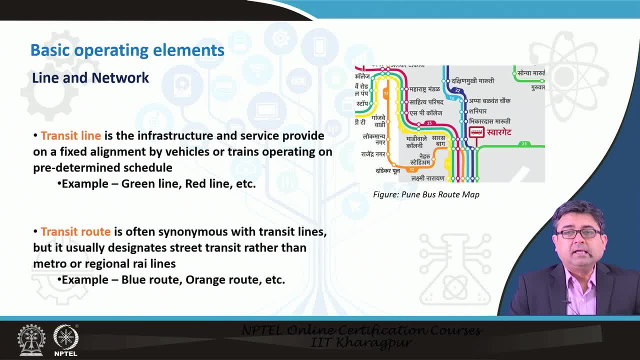 if you had to go from point A to point B, you would pick a line given other characteristics of that line. So that is basically what we call as a transit line, and sometimes transit line and transit route are synonymous to each other, ah, whereas a transit route usually. 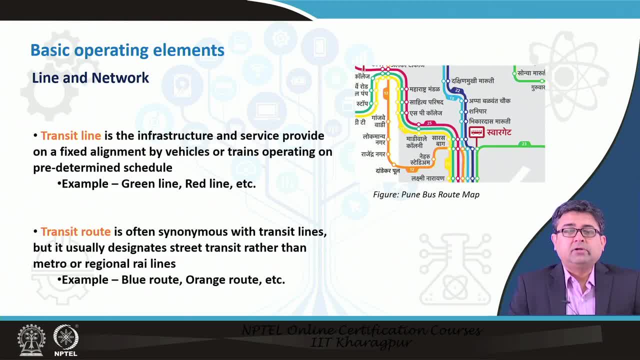 ah designates street transit rather than metro or regional rail lines. So street transit, meaning they have to be operating. if they operate along with other transportation modes, such as cars and auto rickshaws and so on and so forth, then they are called street transit. 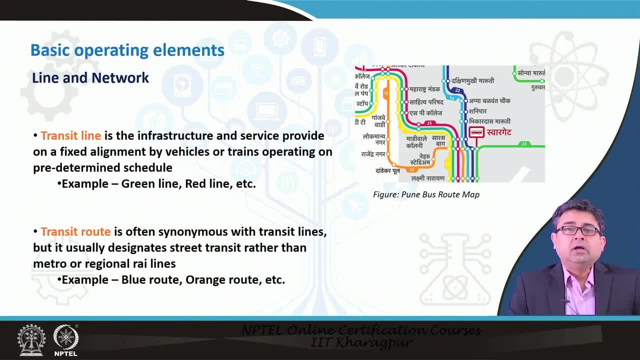 So when it comes to street transit transit, we call it transit route, ah, rather than a transit line. So, in the same example, if it is a bus route, so ah, we will call it. these are all the different routes, so blue route, orange route, and so on and so forth. 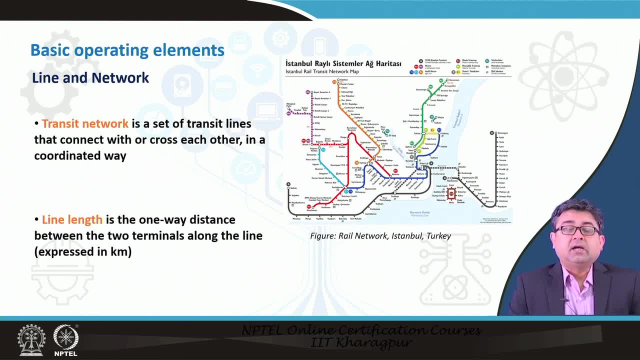 The next terminology to remember is a transit network. So there may be different lines, there may be different routes in a public transportation system, and what a transit network says is that it transit network is a set of transit lines that connect with or cross each. 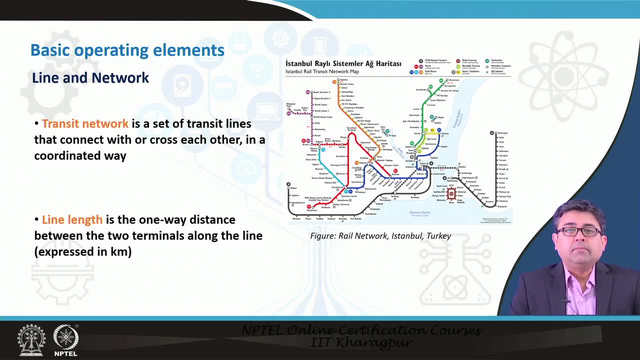 other in a coordinated way. So the transit network comprises of several transit lines or transit routes. So here you would see again a map of the rail transit network in Istanbul, in Turkey. So you would see that there are several transit lines, some of the 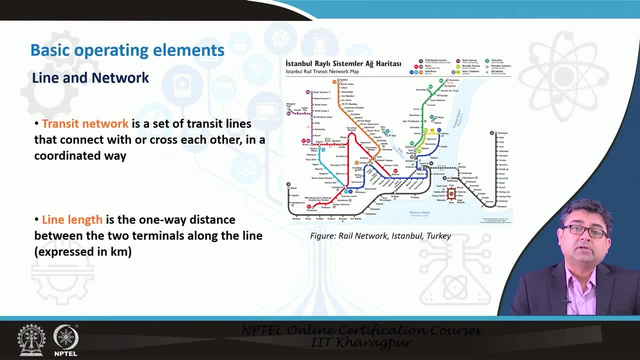 lines run parallel to each other, whereas some crisscross. So the crisscross is by design. ok, So crisscross is not accidental or due to, ah, different alignments coming ah, to meet at one point, but they are actually designed. 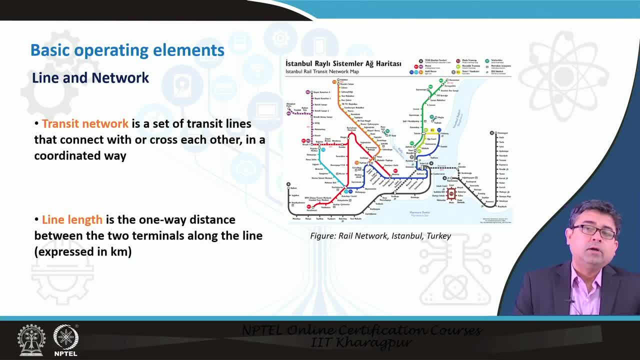 in such a way that people can move efficiently from one point to the other in the city. So that is what is a transit network. So all of these lines collectively would represent a transit network. Then the next terminology to remember is line length. So when we have so many transit lines, we have to remember what is the length. 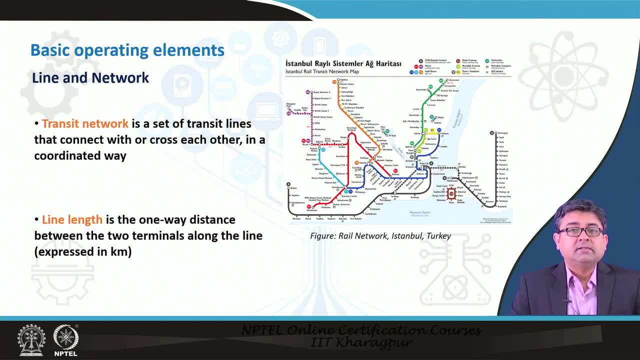 of a particular line. So line length is defined as the one-way distance between the two terminals along the line, usually expressed in kilometers or miles of whatever the unit is. So if you look at ah this map, you would see a black line at the bottom of the ah map which runs 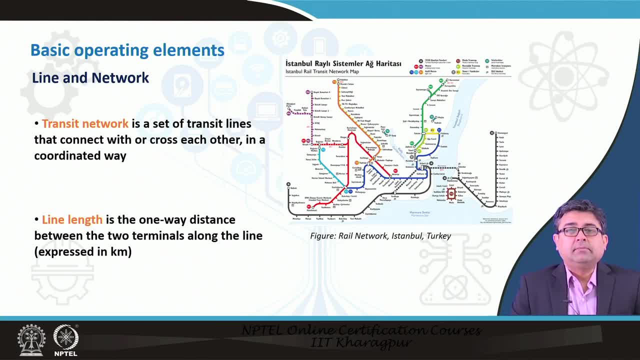 from point ah in the western, ah westernmost point or an easternmost point, and vice versa. So you you can call that ah or you can calculate the line length of the black line from the terminal that is in the easternmost side to the terminal at the westernmost side. So 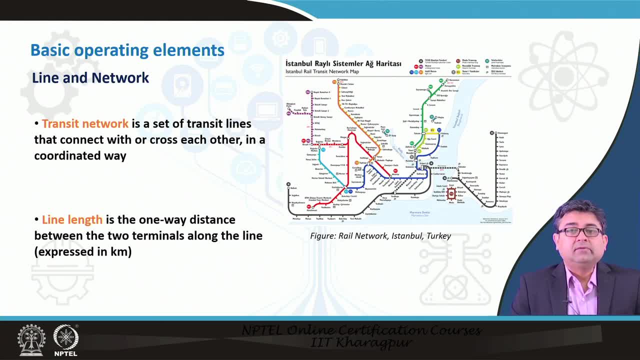 between the two terminals. the entire length, length of the line is called the line length. So this, these are all operational ah terminologies that help in scheduling a bus service or a rail service. So once you know that your transit line is n kilometers long and you 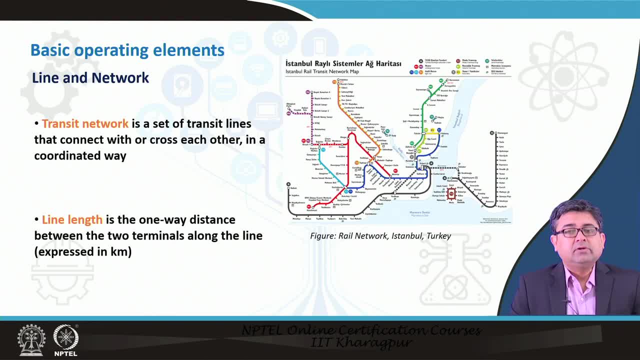 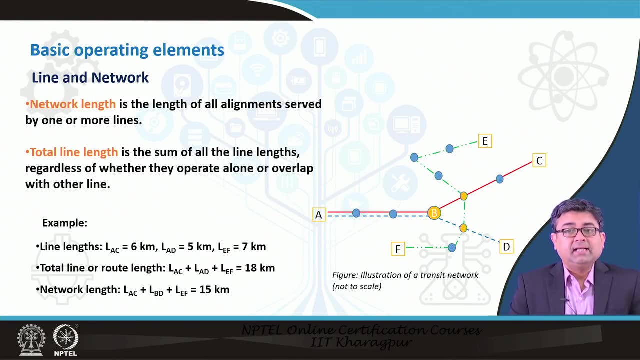 have s number of stations in between, So you can then schedule your transit ah line accordingly. So moving on, next is what is called the network length. So now you know the line length. So, in similar way, you have to now determine what is the entire length of. 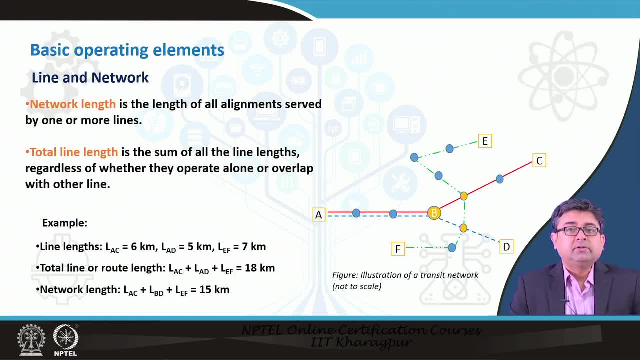 your network, that is, within, within the city. So the network length is intuitive and easy to define. is the length of all alignments served by one or more lines, So you have multiple lines. then what is the length of all of those lines added together? 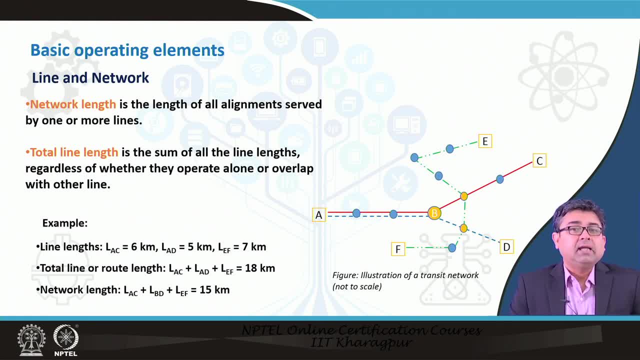 A similar sort of a ah terminology is called total line length and we will see how it is different from ah, network length, ah in the example, ah that is following this definition. So total line length is the sum of all the line lengths, regardless of whether they operate. 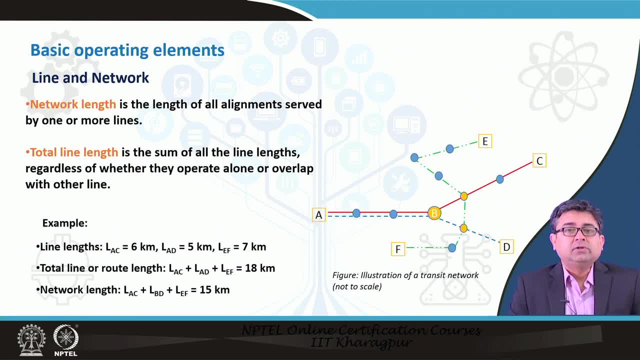 alone or overlap with each other. So there may be some overlapping ah, ah lines. however, when we consider, when we calculate the total line length, we will calculate all those overlapping lengths as well, Whereas when we look at network length, we usually do not consider the overlapping lengths. 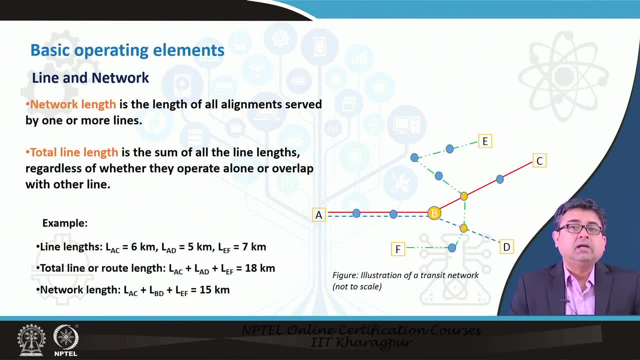 So that is the difference, subtle difference between a network length and a total line length. So here, in this example, you would see that there are: ah, essentially there is a. there is a red line going from terminal A to terminal C. there is a green line going from terminal. 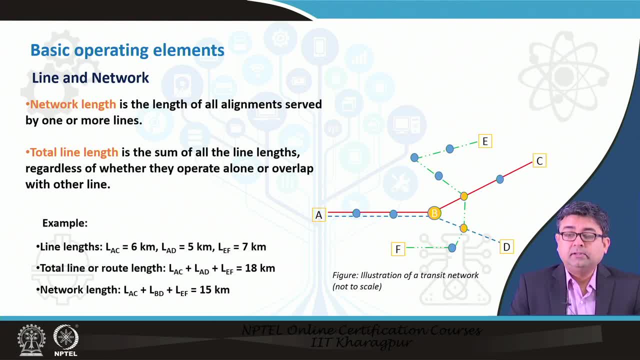 E to terminal F, and then there is another blue line that also starts from terminal A but goes to terminal D. So there are these essentially three lines, but they are criss crossing at different points. So if you were to calculate the line lengths, the individual line lengths, then you would. 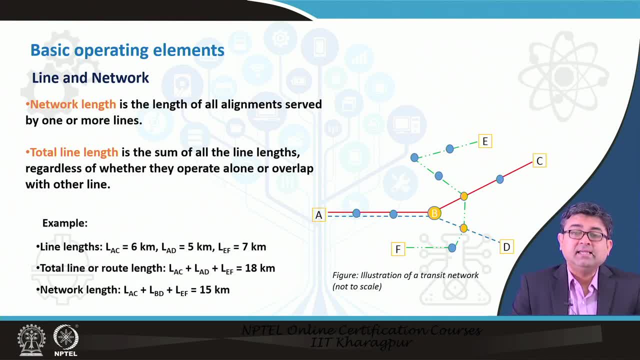 say that ah, line length AC for the line, for the red line, the line length would be 6 kilometers, given that. So every station is equally spaced and it is 1 kilometer each. So if you see, ah, if you see, then you could calculate that the line length AC is 6 kilometers. 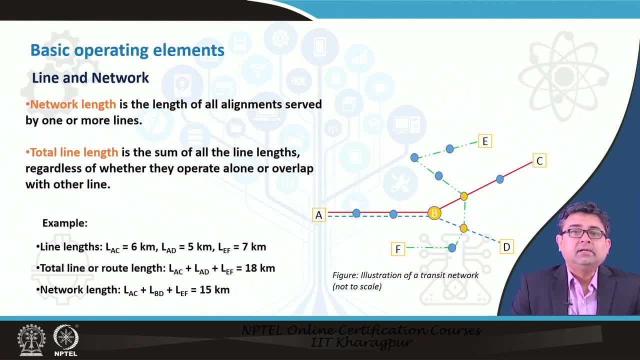 Similarly, the line length AD, which is the blue line, is 5 kilometers and the line length EF is 7 kilometers. So now, when we want to determine the total line ah line length or the root length, what we do is we add up all of these line lengths. 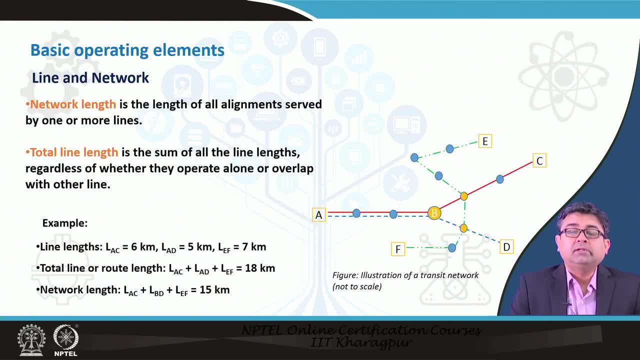 So, irrespective of whether these two lines, which is the red line and the blue line, that are overlapping for one stretch between A and B, we still add all those lines up and say that the total ah line length, or the root length, is 18 kilometers. 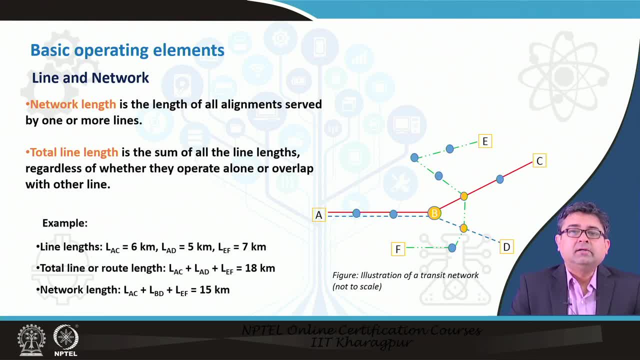 Whereas when we look at the network length, you will see that we are adding AC, we are adding EF, but now we are not adding AD, but we are only adding BD. So so we are neglecting or we are not adding the overlapping section and we are only adding the section that is. 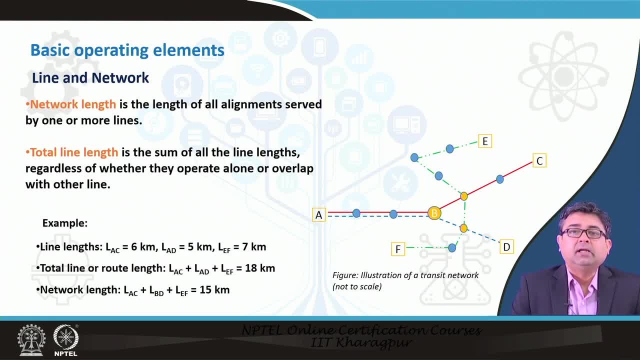 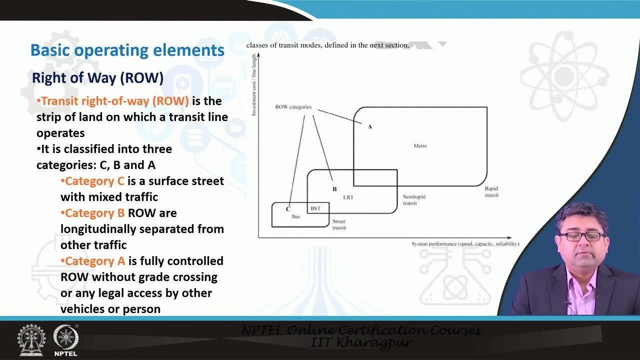 not overlapped. So then we get a network length of 15 kilometers. Hopefully that is clear now. we move ahead Now when it comes to The traffic and the transit runs on that surface street itself. ok, 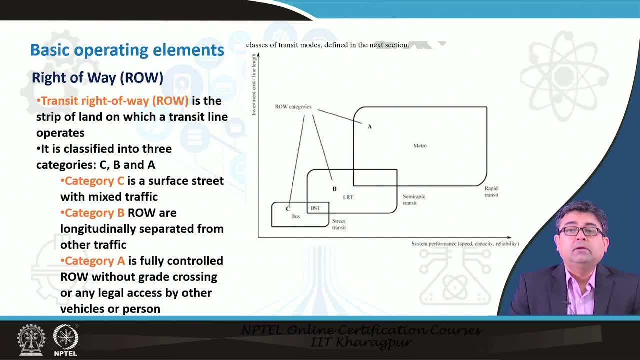 So category C is a surface street with mixed traffic, So that if there is that kind of a right of way, then we say that this is a category C right of way, Whereas when the right of way are longitudinally separated from other traffic we call them. 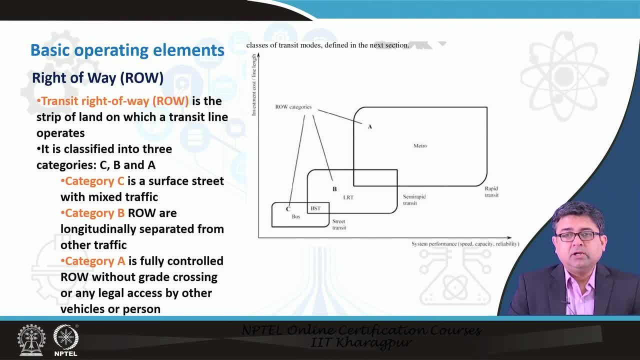 as category B. So what do we mean by longitudinally separated? So maybe there are, ah, there is a median on which ah A public transportation line runs, So the median is separated from the ah adjacent ah vehicular traffic by some sort of a tree. 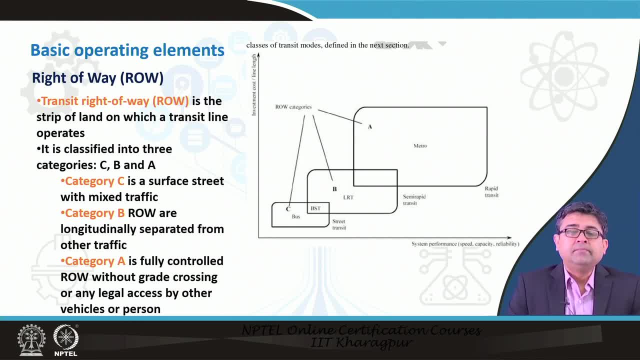 line or some sort of a different pavement type. So that is, but they are still running on the surface. the transit line is still running on the surface. So such type of right of ways are categorized as category B right of ways, whereas category 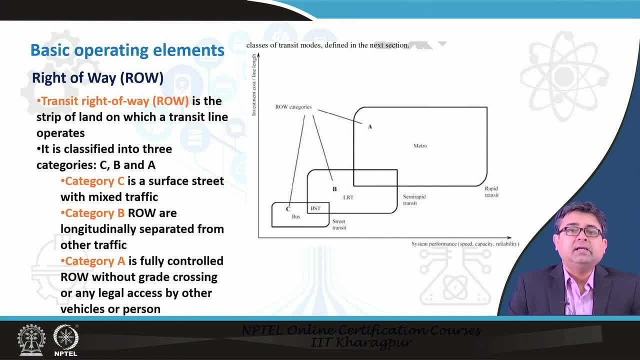 A right of way is a fully controlled right of way And without any grade, crossing or any legal access by other vehicles or person. So when we see the metro lines usually that are over ground or above ground, such kind of right of way for the transit or public transportation is categorized as category. 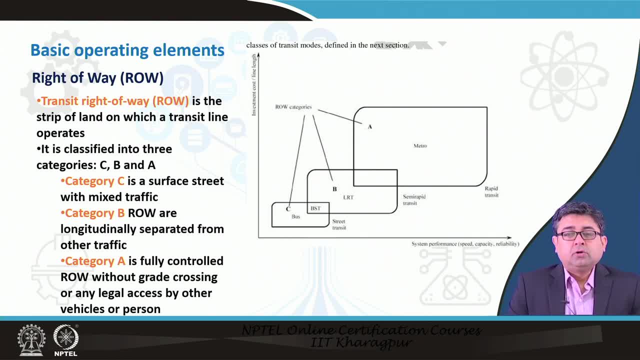 A public transportation. So, ah, category, A right of way, sorry, Ah. Now, if you look at this chart, and ah, we would not go in detail, ah, in this chart, but you can see that there is a right of way In this chart, but ah, that we would do it later, but this, you would see that ah the. 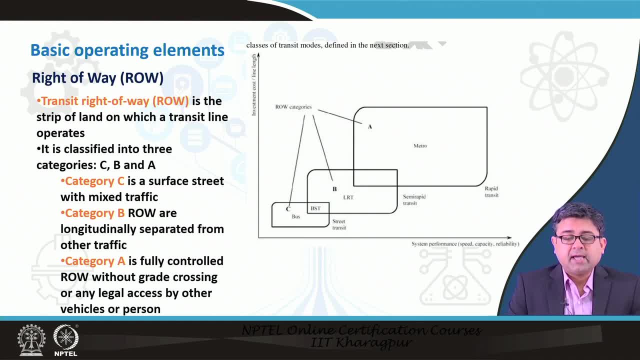 x axis has the system performance, whereas the y axis has the investment cost per line length of any system. So you would see that if it is category C type of ah, right of way for any public transit, you would see that the cost is very low, the investment cost. 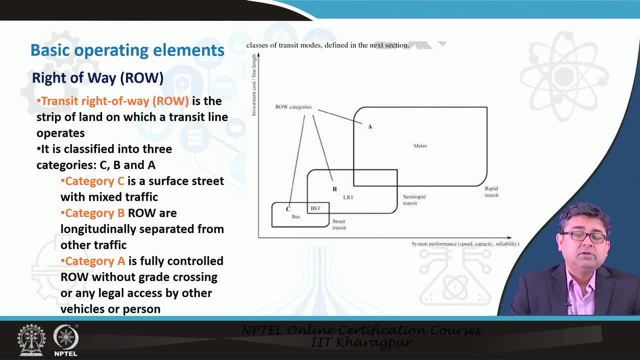 is very low, but the system performance is low as well. So to introduce ah- in other words, we can say that to introduce a bus transportation ah in any city. it may cost ah very less, but at the same time the system performance. 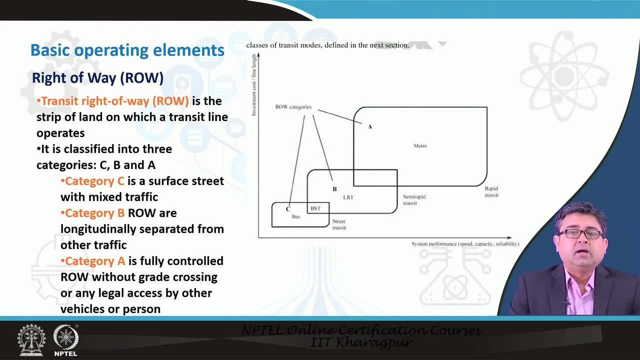 would also be very less. What do we mean by system performance? Ah, Schedule, ah, staying on schedule, staying on time, all of those things, and we will look at it in much more detail later on. So, similarly, now, if you move on to right of way type B, the cost. 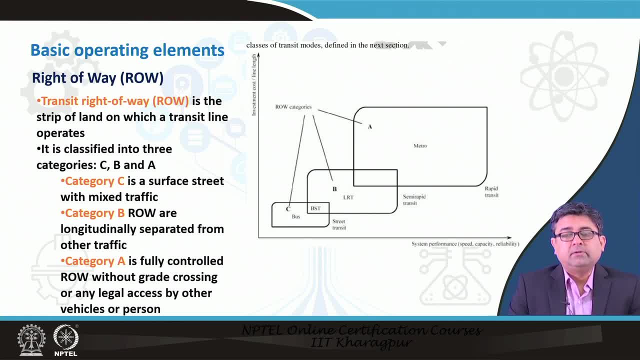 increases a little bit as well, as the performance also increases. However, then, when we finally move on to right of way, category A, that has the largest cost and the most ah good, ah, system performance as well, And the breadth, ah, the breadth of the boxes say that what is the? 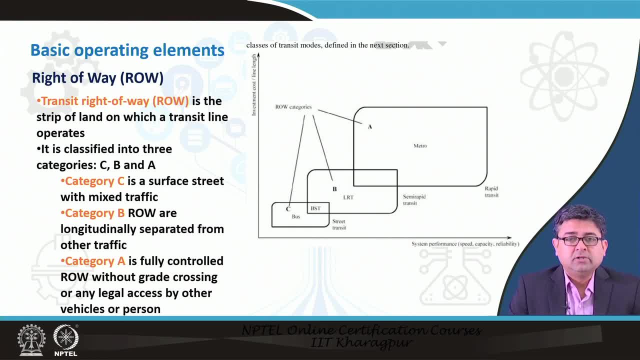 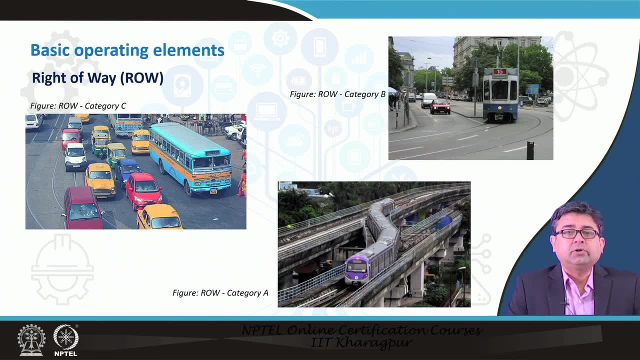 range in the system performance and the range in the costs. So that is, and that kind of gives you an idea of how the right of ways are categorized. If I wanted to show it in pictures, you would see that the first picture on your left is. 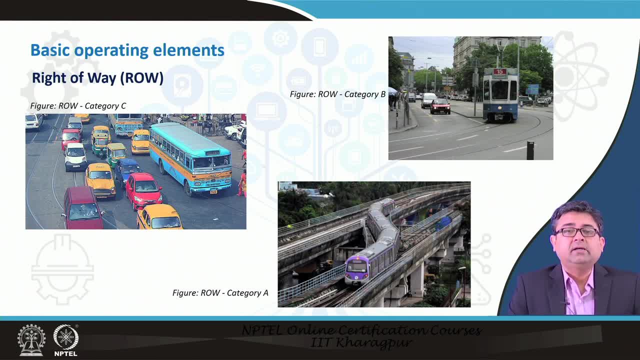 a right of way. category C, where the bus is travelling along with all the other vehicles on the street. Ah, If you move, ah, anti or clockwise, to category B, ah, that is the picture of a tram which has its own right of way, So it has its rails. that has, that is, that is its own right of way, but the rails are. 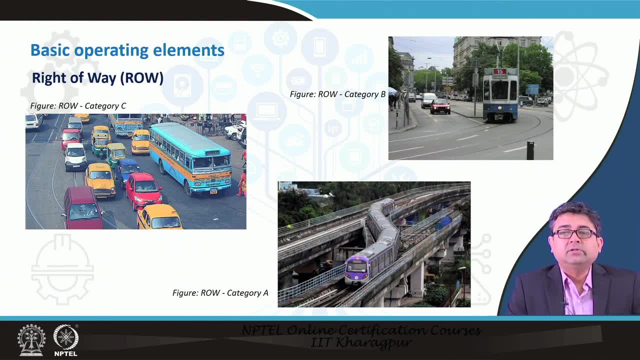 right At grade with the other modes of transportation. So, although it it has- ah, it has- its own right of way, but it is running with mixed traffic, Whereas when it comes to category A right of way, they are usually the metro systems or the subway systems across various 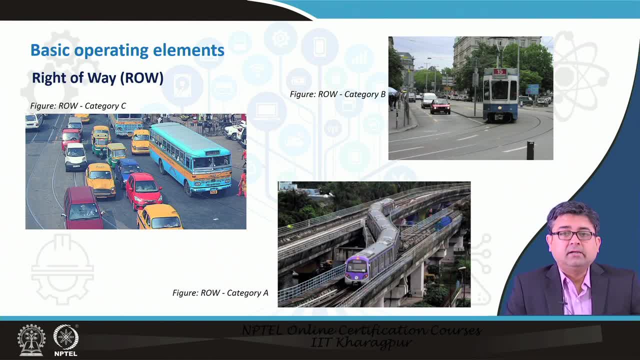 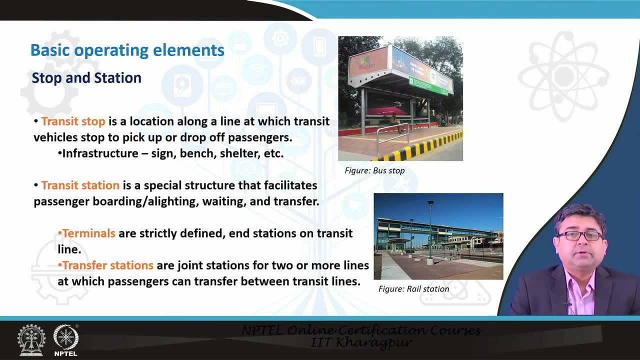 cities in the world that have category A right of way. Now let us move on to the other types of operating elements that are ah involved in public transportation and which you had to ah which you have to know. If the first thing is a transit stop, So we all ah go to a designated place on, ah on. 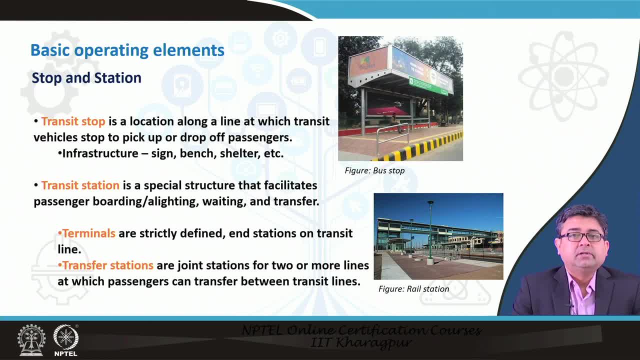 the road to avail any type of public transportation. So transit stop is a location along a line which transit vehicles stop to pick up or drop off passengers Easy enough. this can be easily identified by various infrastructures that are in place at these locations. 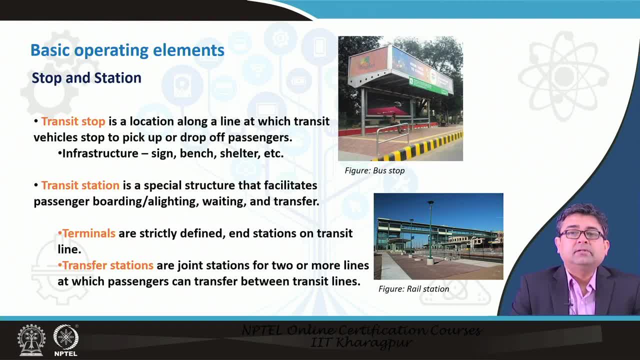 Such as sign benches, shelters, etcetera, and a picture on the top is illustrating the same. A transit stop and a transit station are, ah, synonymous to each other in the way that both of these are locations where they transit vehicles, pick up or drop off passengers, But a transit station is a special structure that 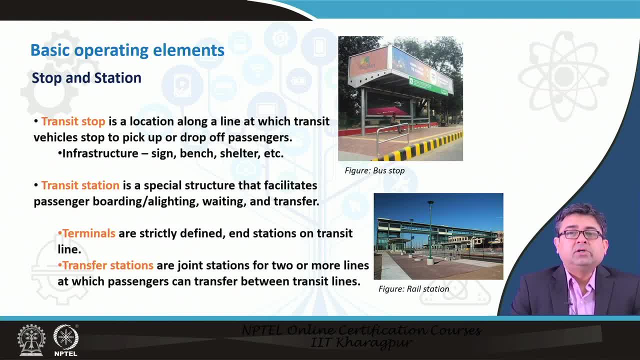 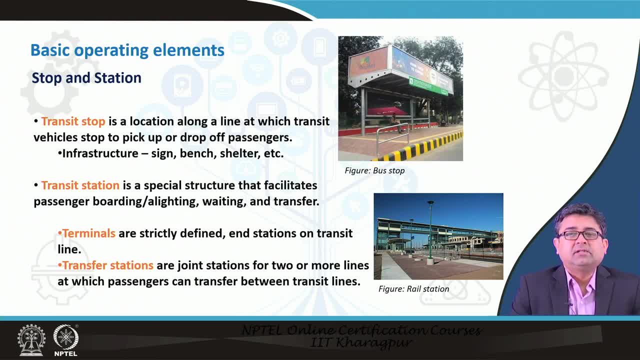 So it is a transit station. So it is a transit station In ah, in a line, whereas the transit station could be a linear feature along that line. So it has some ah, more sitting facilities. It has a variable information available. ah, It, it is. ah, it requires a little bit more. 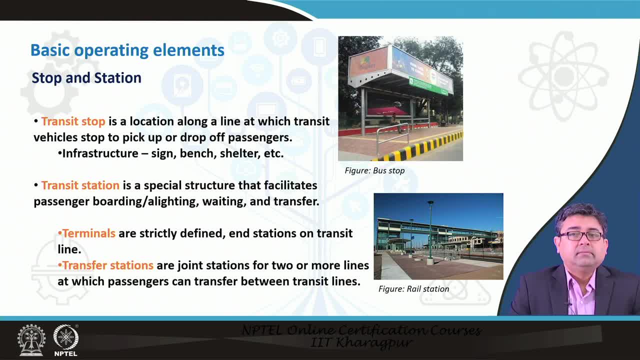 infrastructure to actually accommodate the public transportation vehicles and usually ah we call ah if they are Rail Public Transportation Systems and we usually call those stops as transit stations, ah, whereas if it is a more rubber, tired or bus type of public transportation system, we call those kind of ah stops as transit stops. So both of them are similar, but just. 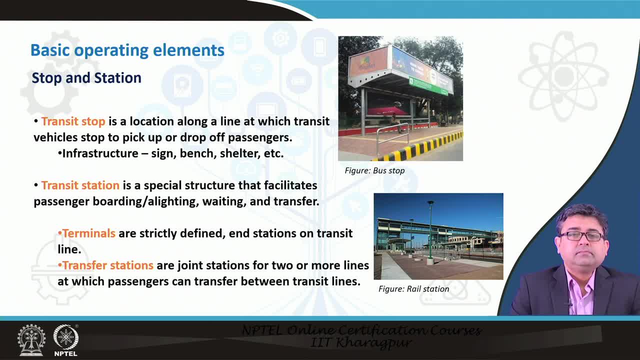 a little bit of difference in terminologies Now. ah, when we look at transit stations, they may be two different types: one is a terminal station and one is a transfer station. So terminal stations are strictly defined and stations on the transit line end stations. 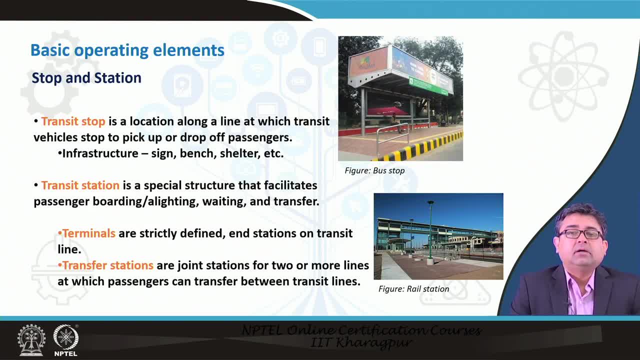 on the transit line. So, like we looked at the ah ah map earlier of the ah rail transportation network in Istanbul, Turkey, So along those black routes, along the black line length, along the black line transit line, we saw two terminals, one on the east. 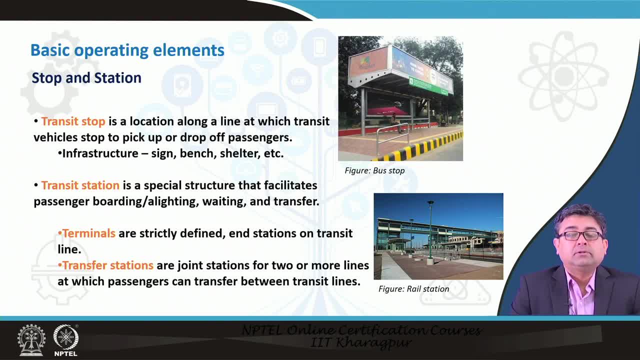 and the one on the west. So those two terminal, ah, those two stations are, or stops are called as terminal stations, whereas there may be other stations where people could transfer from the black line, for example, to the other green or blue lines. So such 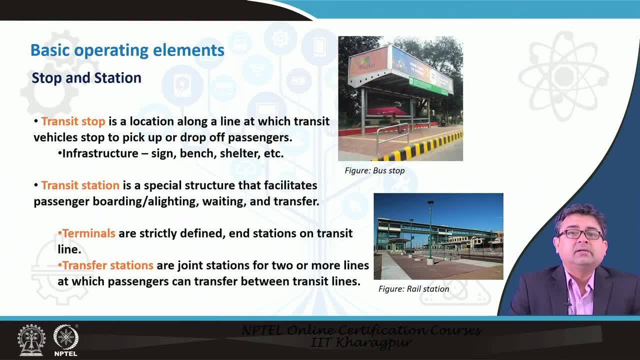 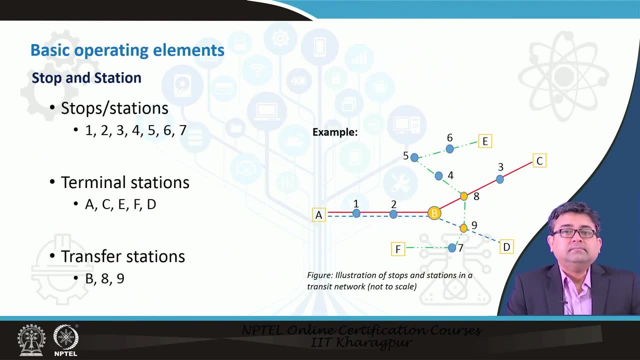 stations are called transfer stations and they are joint stations for two or more lines at which passengers can transfer between transit lines. So a transit station could have two different classifications as well. So if you go back to our ah sketch of the transit route network, we would see that stops or station numbers 1,, 2,, 3,, 4,, 5,, 6, and 7. 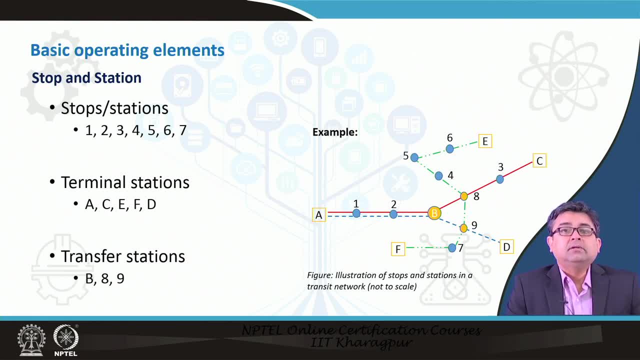 could be called stops or stations. So all the blue dots and the two small orange dots- not the two small orange dot, but all the blue dots- could be called as stops or stations, Whereas the terminal stations are the ones ah, noted in square and has an alphabet inside. 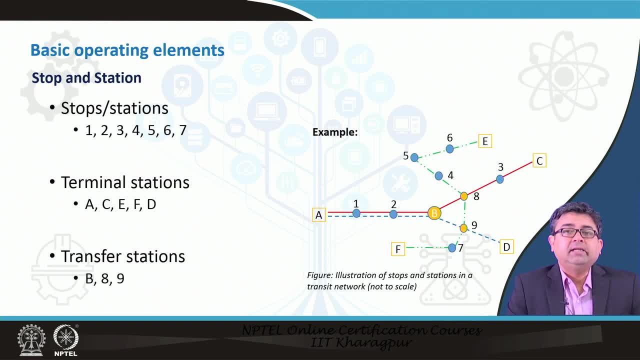 the square. So A, C, E, F, D. So these are the terminal stations. So you will see that they are the end of any particular line, Whereas the transfer stations are the ones where people could transfer from one line to the other. For example, the station B is a transfer line. 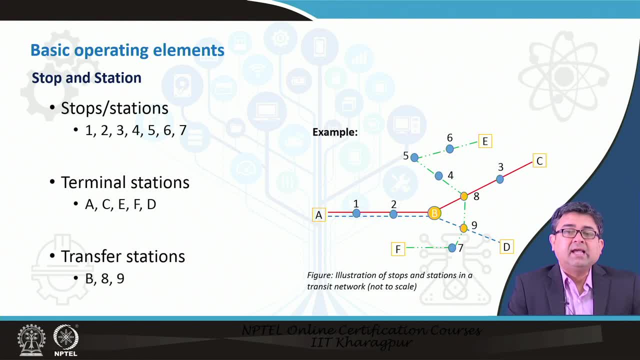 the station 8 is a transfer line, station 9 is a transfer line. So on stations, on station 8, one could transfer from the green line to the red line, Whereas on the ah on station 9, one could transfer from the green line to the blue line. and on transfer ah and on 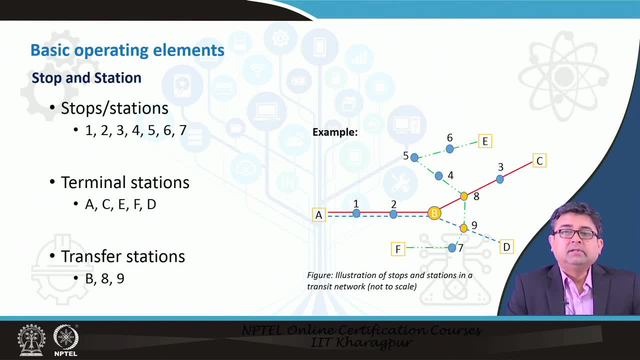 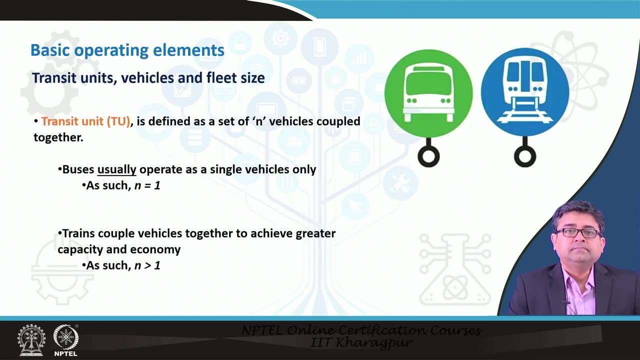 station B, one could transfer From either the red line to the blue line or vice versa. ok, So that is a graphical example of what do we mean by different types of stops and stations. Now the next thing to know is about the vehicles and the transit units and a fleet size. So 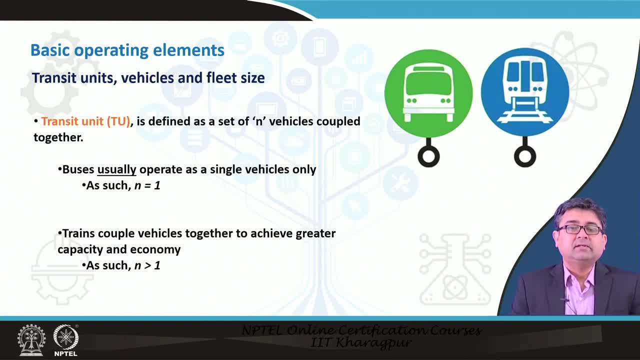 transit unit is defined as a set of n vehicles coupled together. So this is the basic definition of transit unit. when we talk about any public transportation system, It it is called TU in short. So transit unit is defined as set of n vehicles coupled together. Now buses. 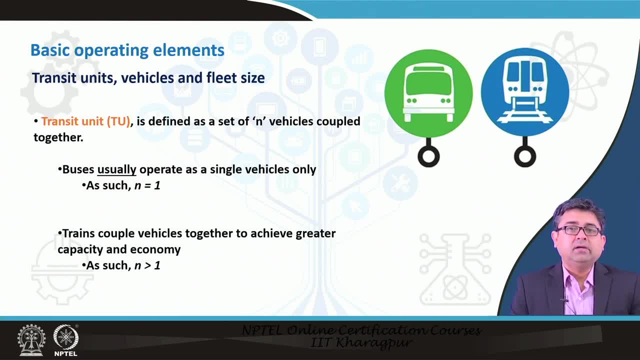 usually operate as single vehicles, So in this case n will be 1,, whereas trains are coupled together to achieve greater capacity and economy, and in that case n is greater than 1.. So now you understand what is a transit unit. Now there are newer buses. ah, that that. 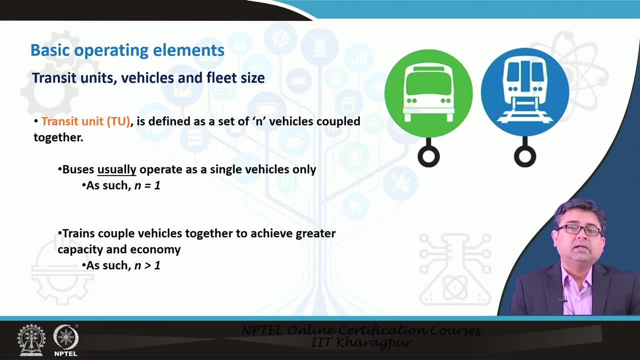 are called articulated buses that may have 2 coaches that are combined with each other. in that case n would be equal to 2.. That is why here we have underlined that buses usually operate as single vehicles. Nowadays we have newer buses that may have 2 coaches. 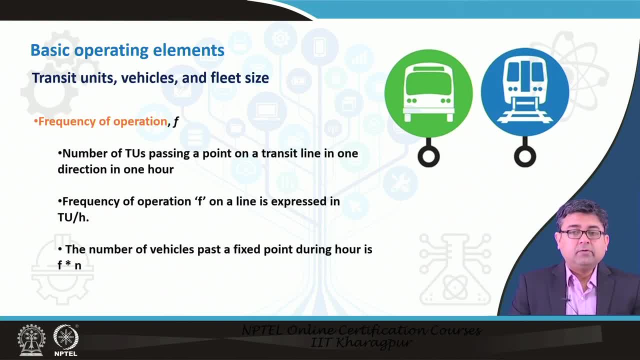 Next is to understand the frequency of operation. Now we, as passengers, are always interested in this frequency. We always want to know When is the next bus coming or when is the next metro rail coming. So how do we operationally define frequency? It is called, as it is defined, as the number of transit units. passing a point, 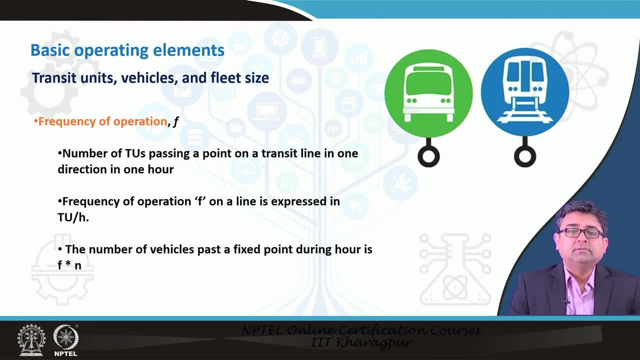 on a transit line in 1 direction in 1 hour. ok, So it is a number of transit units passing a point on a transit line in 1 direction in 1 hour. So the frequency of operation f on a transit line is usually expressed in terms of. 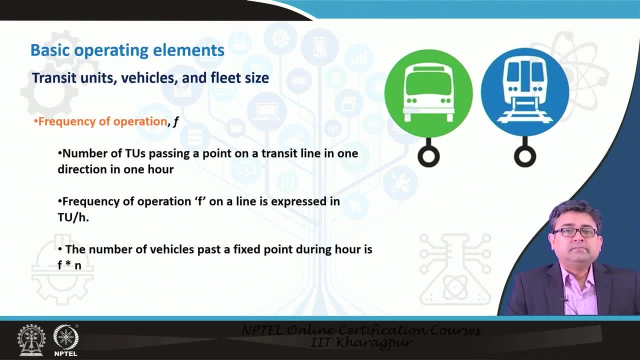 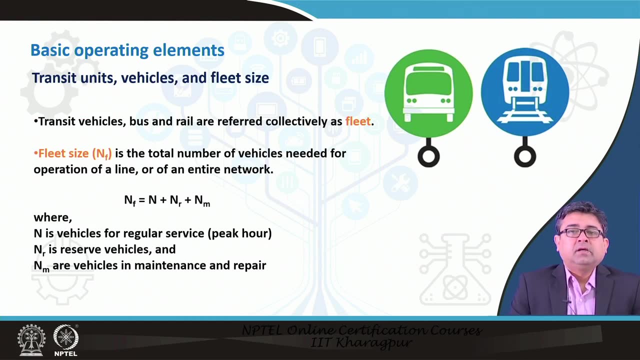 And similarly, if you understand, if you just want to calculate the number of vehicles passing a fixed point, it is f times n, So that is the frequency of operation. Now, when we say fleet, what do we usually mean? So fleet is nothing but a collection. 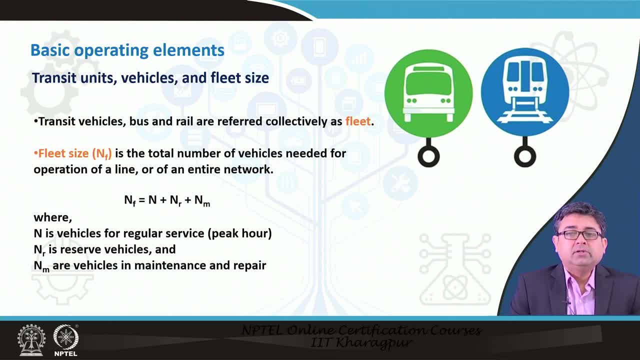 of all the transit vehicles, buses and rails together. So a city, a particular city, may have different types of vehicles that offer public transportation. So you may have buses. you may have some cases in cities like Kolkata. you have different types of buses: mini buses, air conditioned buses and many of the cities also have air 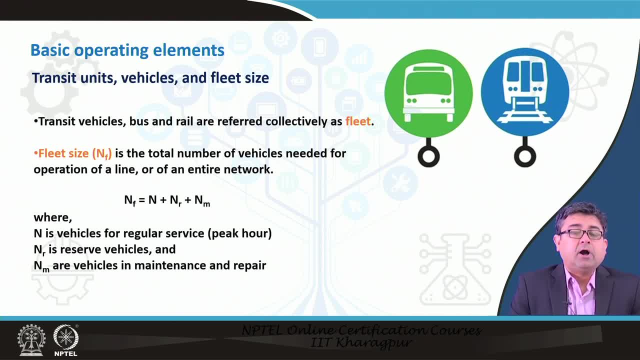 conditioned buses now. So these kind of all of those vehicles, vehicles and buses put together along with the rail, you would collectively call them as fleet. So when we are talking about how efficient is a public transportation network in a, in a city, we usually see what 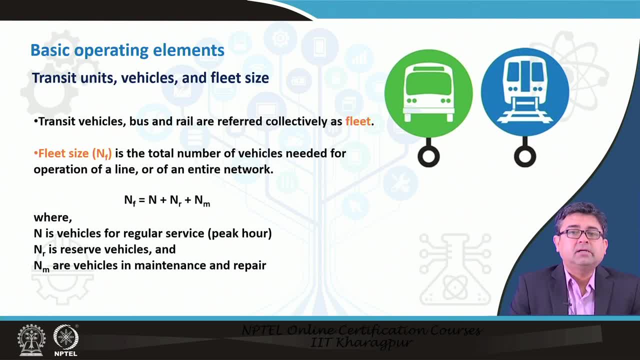 is the fleet size. So all of these vehicles put together, what is the size of the fleet? So the fleet size can also be now calculated as the total number of vehicles needed for operation of a line or of a entire network. ok, 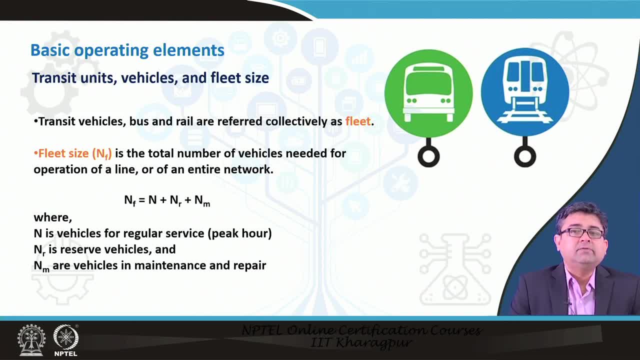 So we have to have a minimum number of fleet size, otherwise we may not be able to meet the demands of the people, People residing in the city. So the fleet size now consists of three different elements. One is the. one is N, which is the vehicles for regular service, So during morning and 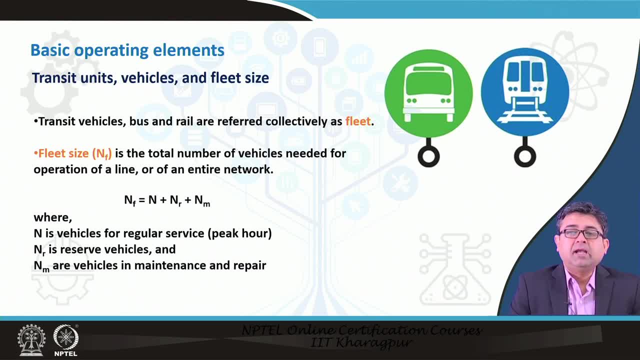 peak hours- morning and evening peak hours- you need N number of vehicles to meet the demands of your citizens in the city. Then comes N F or N R, N, sub R, which is the reserve vehicles. So you always have to have some vehicles reserved in your fleet So that 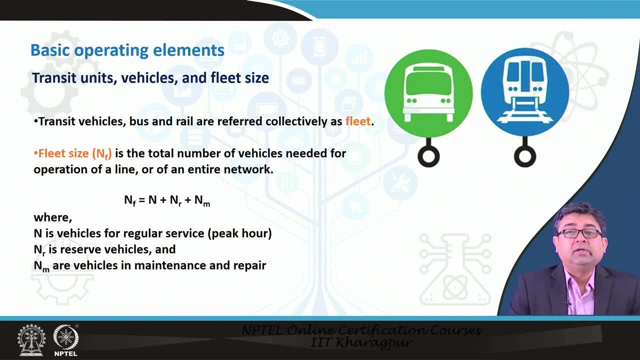 if some other vehicle breaks down or you need additional vehicles to meet additional demand on certain days, you always can use these reserve vehicles. And then there are vehicles which are classified as N sub base. M are vehicles in maintenance or repair. So sometimes when it breaks down there are different vehicles that go into. 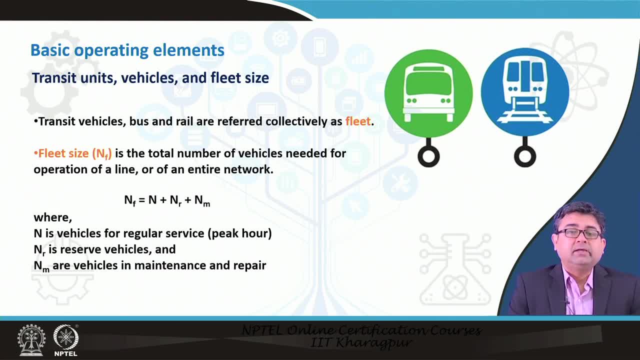 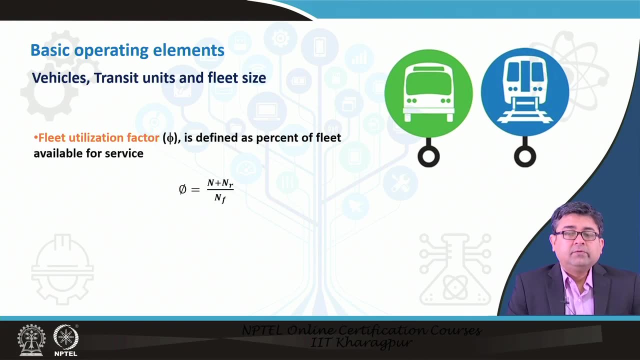 maintenance and repair. So all of these three types of vehicles collectively can be called as fleet size or collectively determine the fleet size. Now there is a terminology called fleet utilization factor, which is usually used by the transit operators and is defined as the percentage of fleet. 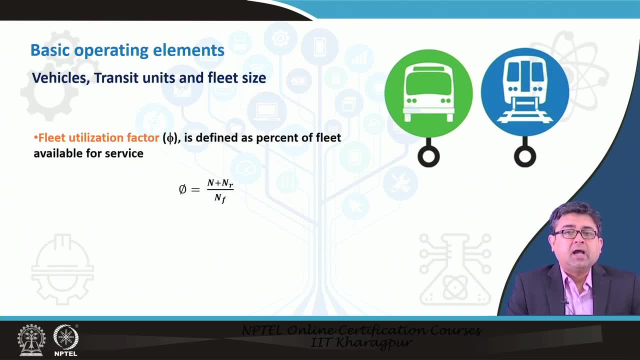 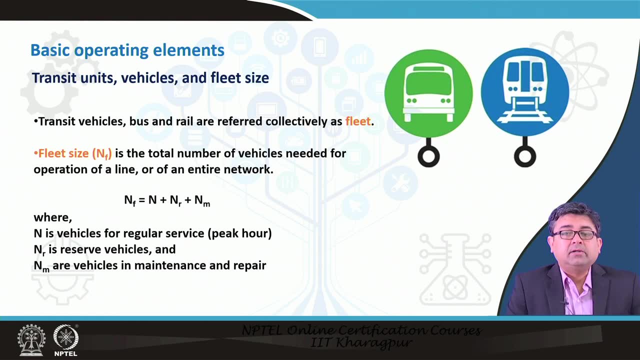 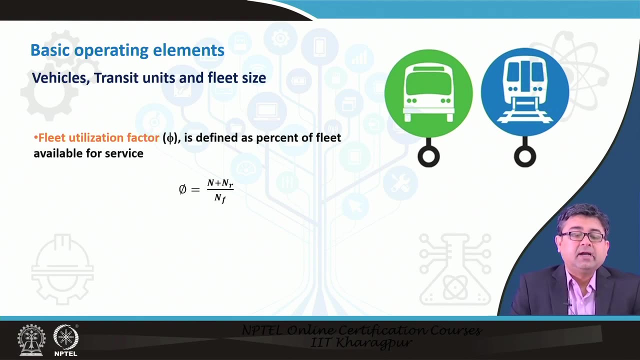 available for service. So, like this, like we saw and in the earlier slide, there may be a lot of vehicles that are available. 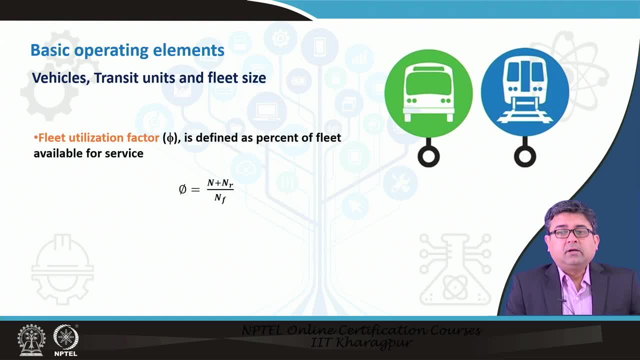 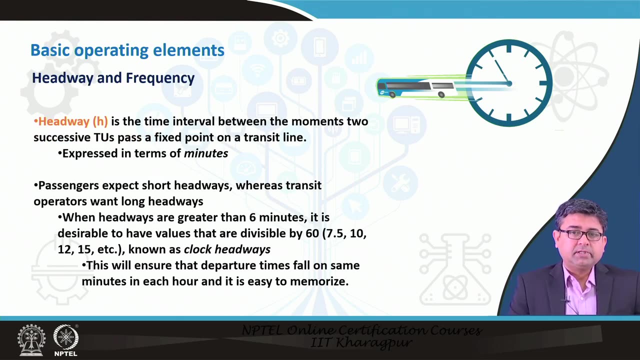 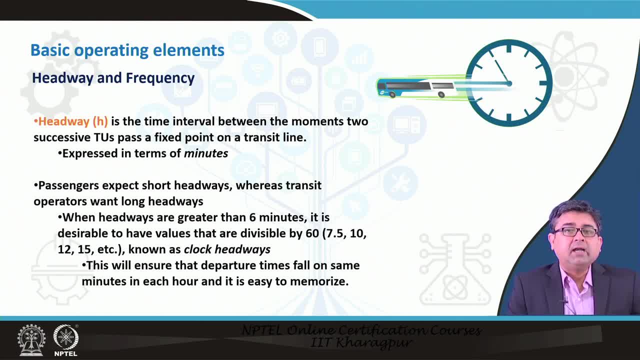 So sometimes we interchangeably use headway and frequency, which have to be ah carefully looked at, they are related to each other. but when we ah interchangeably use it, we may not be doing the correct thing. So headway is. so again, the definition is: 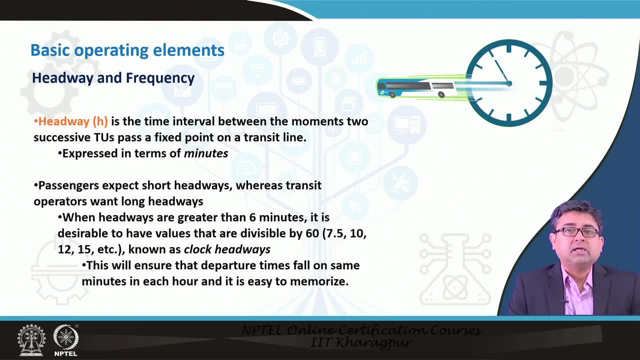 is the time interval between that moments. 2 successive transit units pass a fixed point on a transit line. So there is a transit line which will have lot of ah vehicles. when one vehicle passes a point, the point could be a ah bus stop, and when the next vehicle 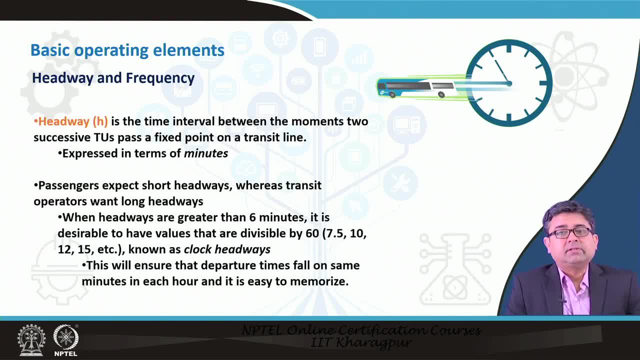 passes that same point on the same line, So the same bus stop on the same line. So the distance between those 2, or the interval between those 2, not not the distance? headway is usually, ah, expressed in terms of minutes, So this will give you the headway. 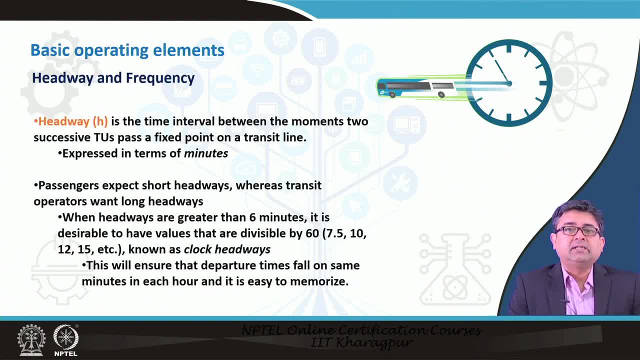 So passengers expect short headways, whereas transit operators want long headways. So we always want the next bus to come very quickly right. So we expect shorter headways, whereas it is very difficult operationally or very expensive operationally to have lot of vehicles. 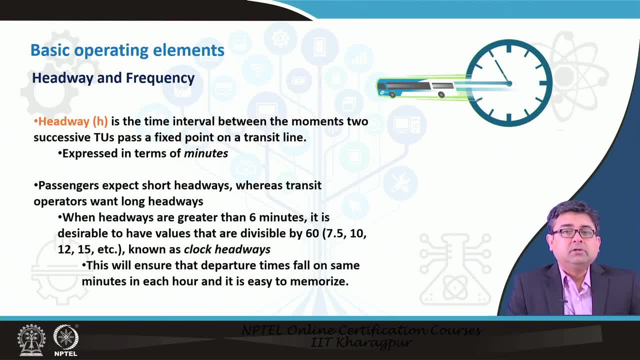 coming in. So usually transit operators want longer headways. So there is a always a give and take and an optimal headway value is usually reached Usually. you would see that if the headways are greater than 6 minutes then ah, it is desirable. 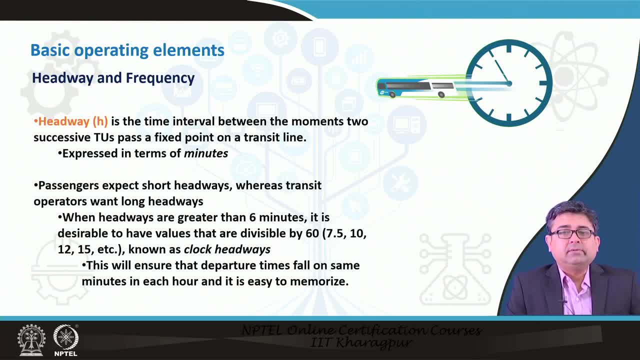 to have values that are can be divided by 60, because an hour has 60 minutes and then you can always remember when the next bus comes. So those are usually called clock headways and it is easy to memorize. So if you divide by 6. So you could say that the 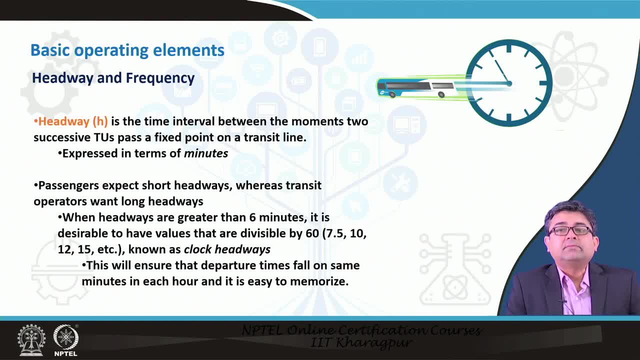 bus comes at ah. 7 minutes past 7 and a half minutes past the hour, 10 minutes past 7 and a half minutes past the hour, 10 minutes past 7 and a half minutes past the hour, 10 minutes past the hour, 12 minutes past the hour, 15 minutes past the hour. So these are usually. 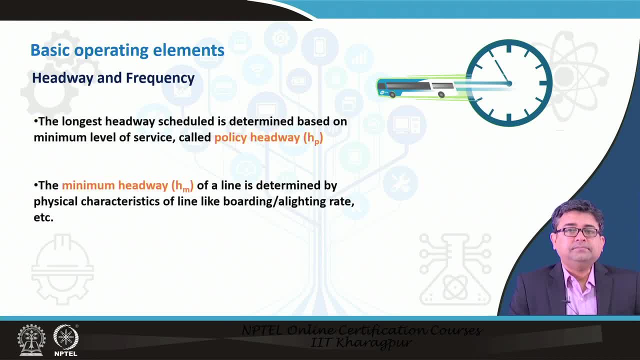 easy to memorize: headways, Something called. there is something called a policy headway which ensures that the longest headway is scheduled, determined based on the minimum level of service provided. Now, since the operator always wants longer headways and ah, users always want shorter headways, So there is always something called a policy. 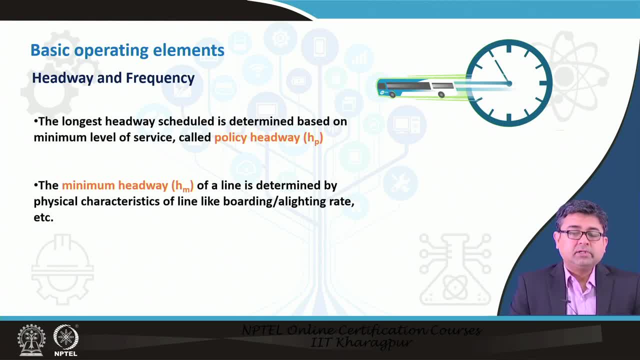 headway That ensures that ah the users are not disgruntled as the. at the same time, the ah operators do not face excessive ah cost in running the transit operations. So there is an headway which is a intermediary point, and it is called a policy headway, which has to be met so that 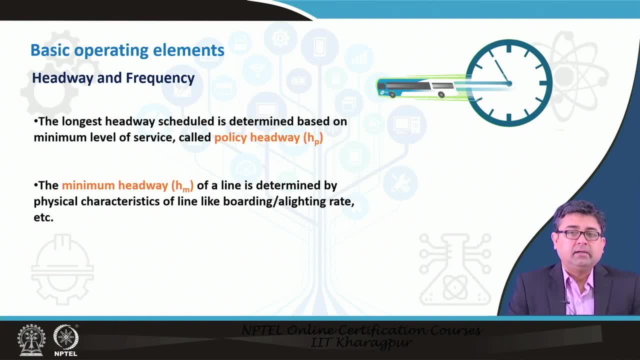 the level of service is, ah, maintained. What is level of service? we will look later on. and then the minimum headway of a line is determined by physical characteristics. So the minimum headway is determined by physical characteristics of the line, like boarding, alighting rate, etcetera. Now there is also a minimum headway that. 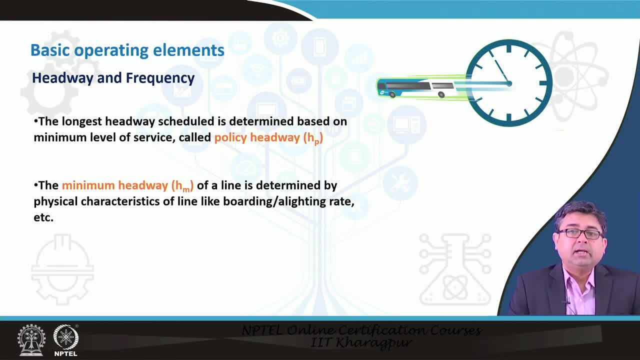 has to be met. ah, and what do you mean by boarding alighting rate? is that if there are lot of passengers boarding or alighting from ah majority of the stops on the line, then it actually affects how quickly a ah vehicle can come and leave that stop. So that will affect. 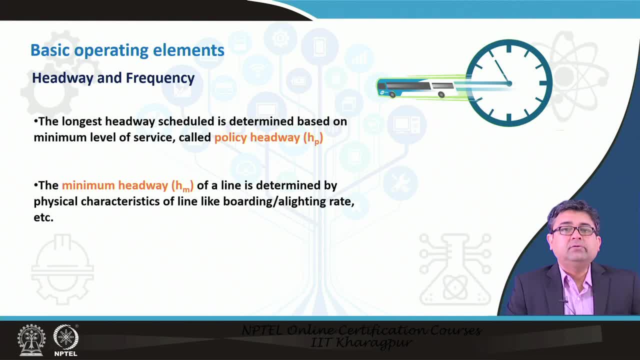 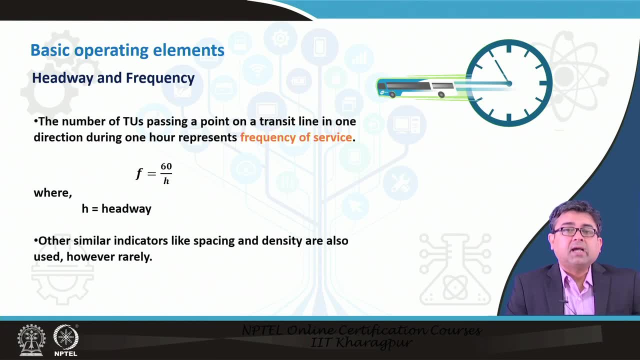 the headways. So there has to be a minimum value that we have to keep in mind. Ah, we have already looked at frequency, but let us look at how frequency and headway are related. So frequency, as we know, is the number of tu's passing a point on a transit. 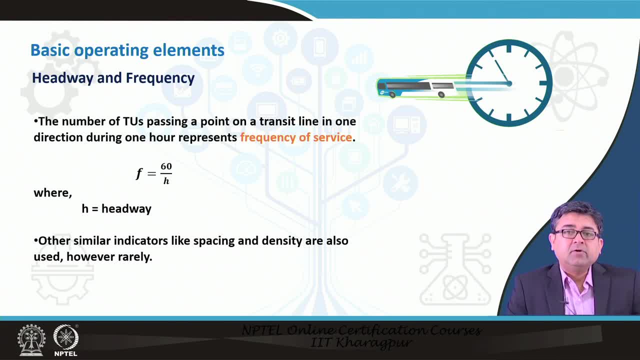 line in one direction in one hour. and here is how frequency and headway are ah related. Frequency and headway are just in the inverse of each other. with 60 divided by h, h is the headway. Sometimes, ah ah. we alternatively use other. 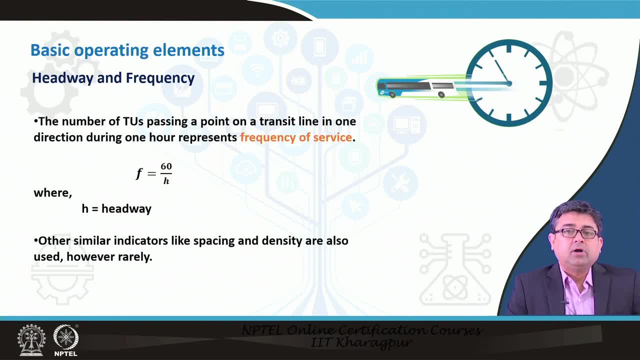 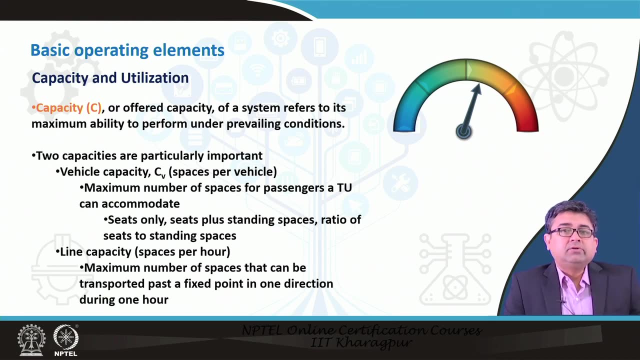 indicators. So instead of frequency we say spacing or density. but ah, frequency is some, is mostly what is used along with headway, but we have to remember the subtle difference between frequency and headway, The last two elements to remember. ah, in this, 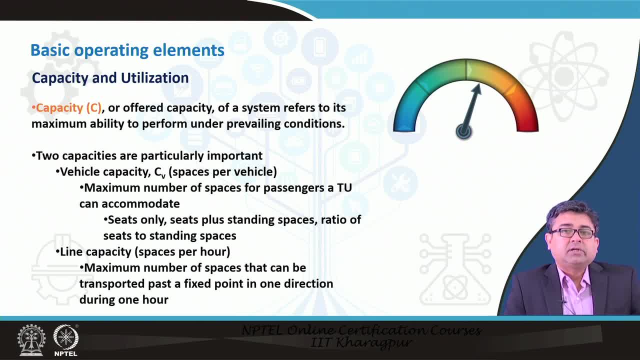 lecture is capacity and utilization. So the capacity or offered capacity of a system referred to its maximum ability to perform under prevailing conditions. So any, any transit line would have a capacity. right. It has a capacity to operate ah n number of ah tu's. it has a capacity to ah ah move n number of people from point A to point B. 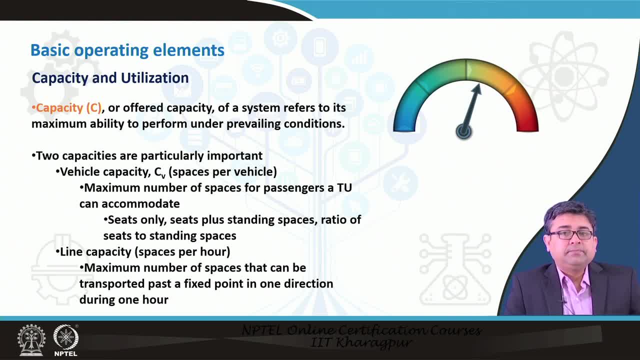 So that is essentially what is called offered capacity. ok, So there are two types of capacities. one is vehicle capacity and the other is line capacity. So the vehicle capacity is the vehicle that is, ah, running on that line. How many spaces are there? How many spaces are? 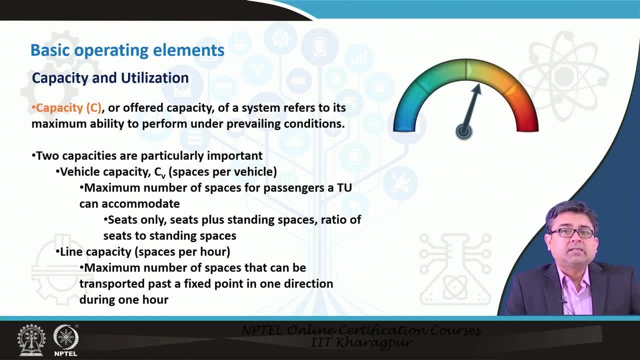 are available in within that vehicle. ok, So the maximum number of spaces for passengers a tu can accommodate. So sometimes we count only the seats, but sometimes we also count the seats plus standing spaces. Sometimes we say the ratio of the seats to standing. 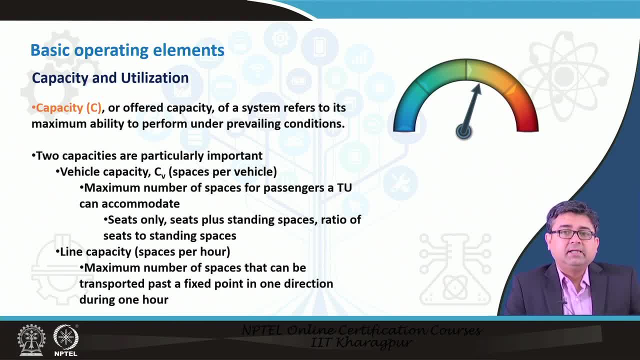 spaces. standing spaces determine what is the vehicle capacity, Whereas the line capacity is the maximum number of spaces that can be transported past a fixed point in one direction during an hour. So there are different types of vehicle capacities. then we can calculate the line. 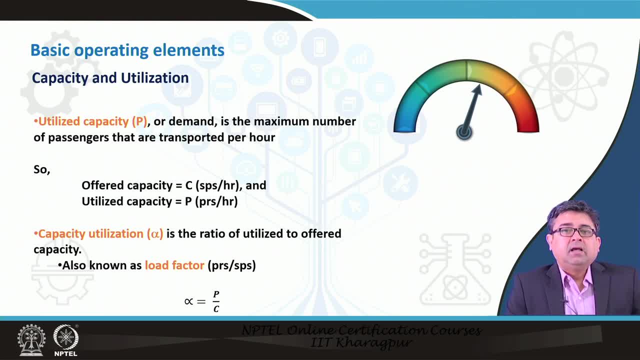 capacity And then the utilized. so these, these two are offered capacities. Now, what is utilized capacity? Utilized capacity is nothing but the demand, which is the maximum number of passengers that are actually transported per hour. So there is always a difference between, ah, what is offered capacity and what is utilized. 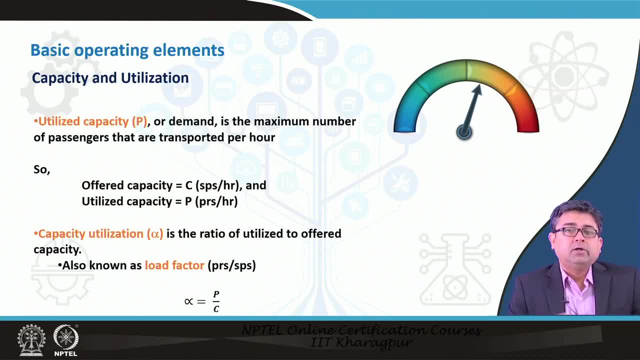 capacity. or, in other sense, there is a difference, but we also want to. So there is a difference, but we also want to keep them close to each other, So we want to keep that ratio, also known as the load factor or the capacity utilization, very close. 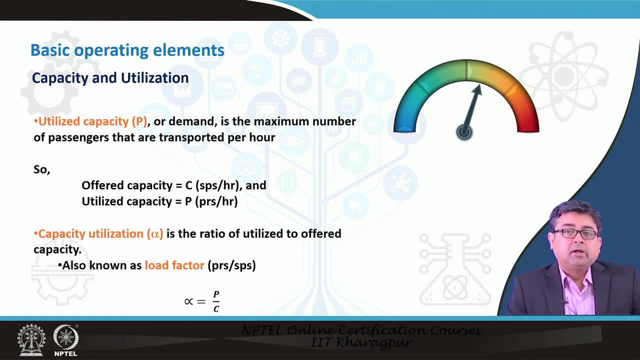 to 1. if it is very close to 1, then we are operating at optimal level of service, Whereas if the offered capacity is very high, ah, whereas the utilized capacity is very low, then we are. the load factor is low. So we understand the difference between offered capacity utilized. 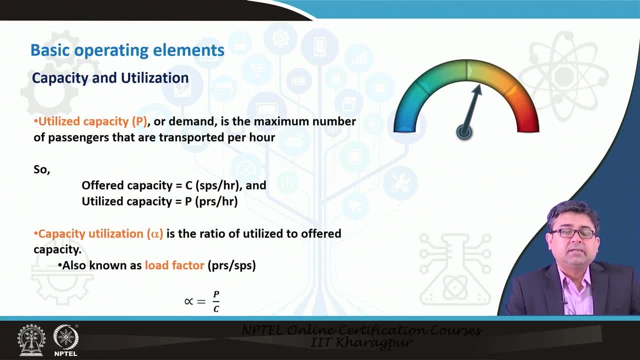 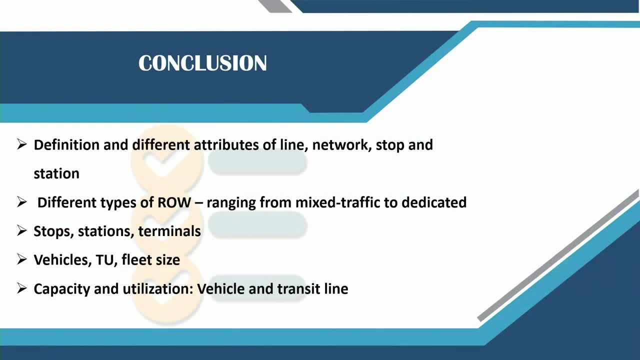 capacity and how both of them are related, is through capacity utilization, which is the ratio of utilized to offered capacity. So, in conclusion, we looked at the different types of lines, network stops and stations. ah, we also made some distinct ah ah distinction between the different types of right of ways, which will allow you to understand how different 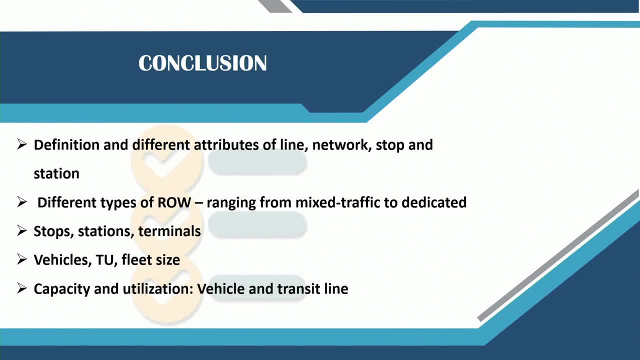 types of public transportations operate ah. We looked at what is the difference between stops and stations ah, how the stations ah differ between ah when they are terminal or when they are transfer stations. We looked at the basic unit ah of transit, which is transit. 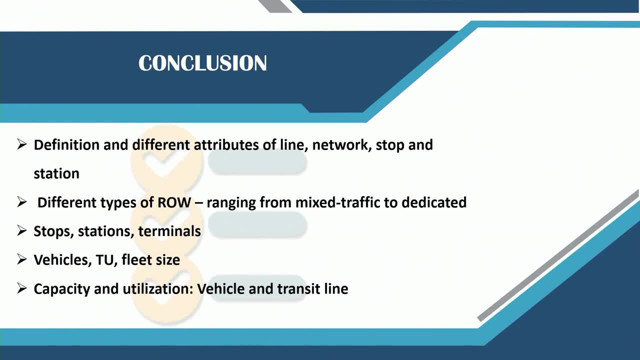 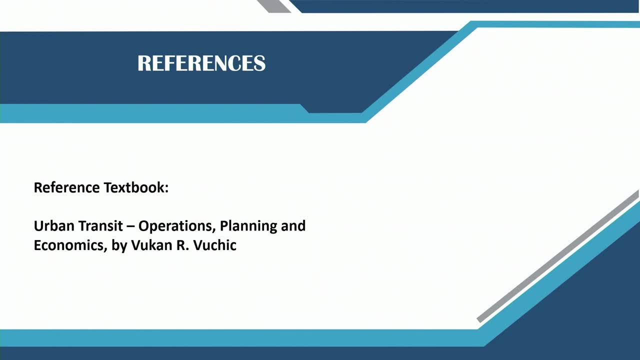 unit TU, looked at fleet size, different vehicles and finally, looked at capacity and utilization. So now, ah, I would like to refer you to this textbook, Ah called Urban Transit Operations: Planning and Economics, by Vukhan Vucic. ah, this would 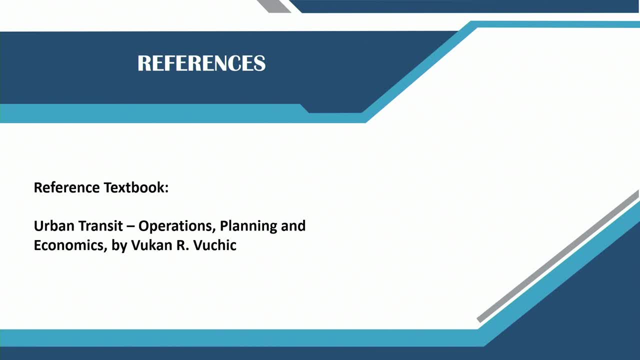 be primarily the textbook that will be ah used for all the lectures on public transportation, and you would find lot of reading material in this textbook, So I would request you all to get it, Thank you.